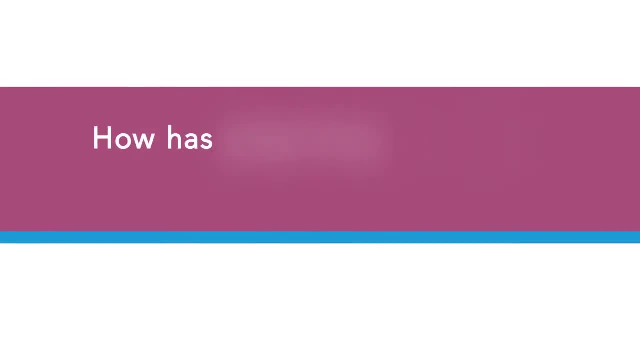 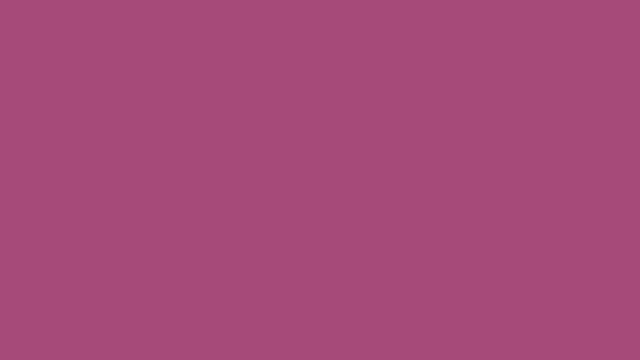 first grade. Let's take a look at how enrollment in pre-primary programs for three to five-year-olds has changed over the years. Overall, pre-primary enrollment has not grown much in recent years, but full-time enrollment has expanded quite a bit Since 1990, we've seen major growth. 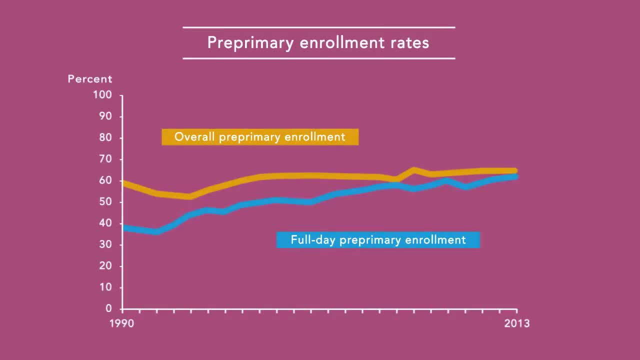 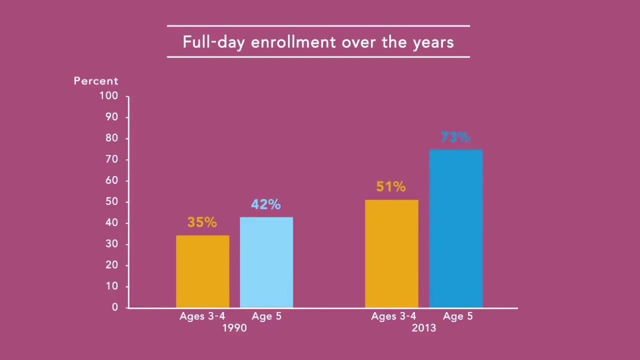 in full-day enrollment, rising from 39% in 1990 to 60% in 2013.. That's a 21 percentage point increase. Growth in full-time enrollment is especially notable for five-year-olds. In 1990, the full-day 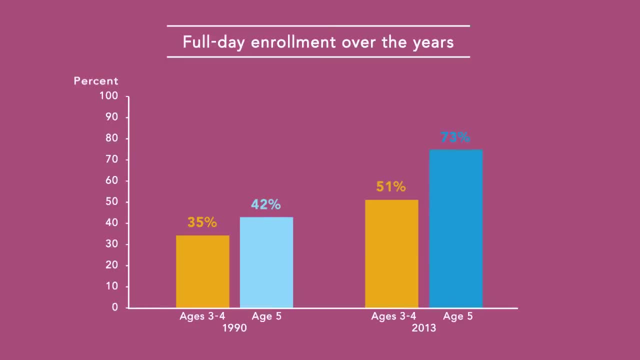 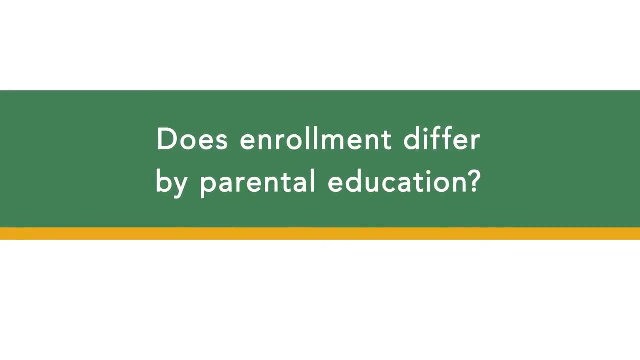 enrollment rate for five-year-olds was only seven percentage points higher than the enrollment rate for three to four-year-olds. By 2013,, the enrollment rate for five-year-olds was 22 percentage points higher. We also find that part-time and full-time enrollment varies by parents' level of education. 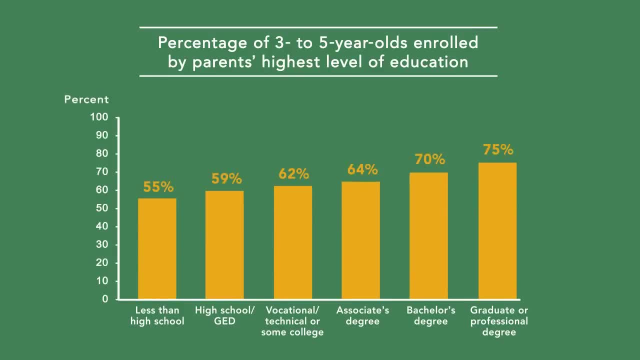 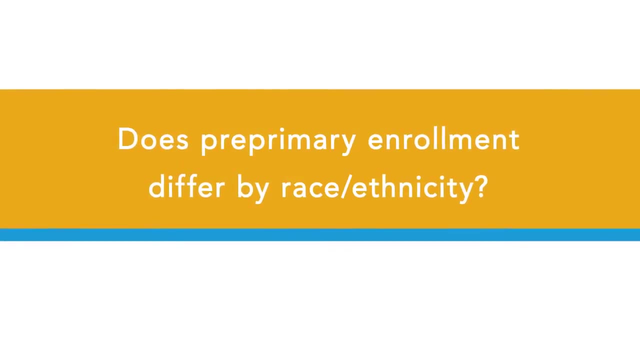 In 2013,, a higher percentage of three to five-year-olds whose parents had a bachelor's or higher degree were enrolled in pre-primary programs than children whose parents had lower levels of educational attainment. Let's see how enrollment rates vary between preschool and kindergarten in the context. 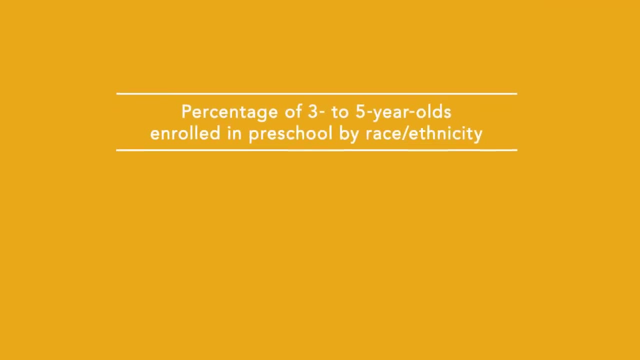 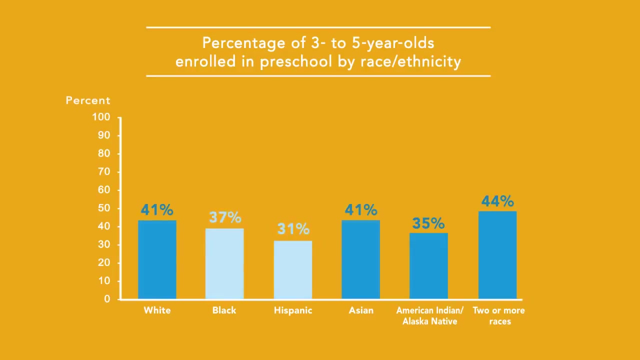 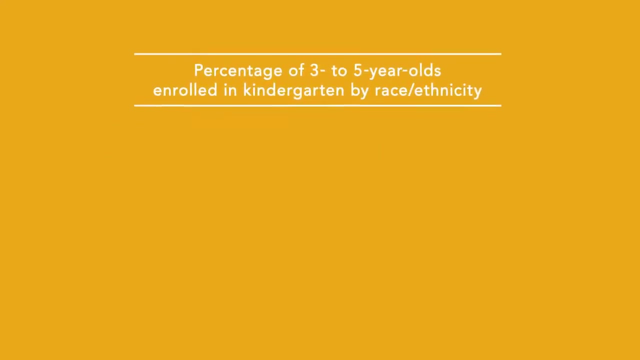 of race and ethnicity. 41% of white and Asian three to five-year-olds were enrolled in preschool programs, compared to 37% in pre-school programs, 37% of black children and 31% of Hispanic children. But kindergarten enrollments tell a different story: A higher percentage of black three. 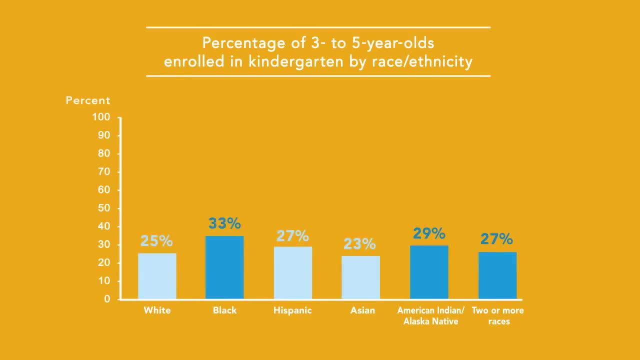 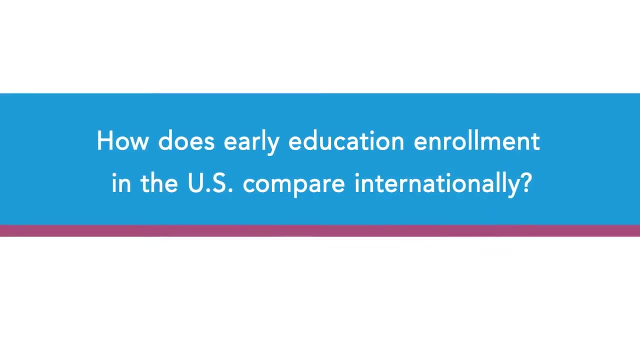 to five-year-olds were enrolled in kindergarten than white, Hispanic and Asian three to five-year-olds. Finally, let's look at how the US compares to other countries In 2012,, among the 34 Organization for Economic Cooperation and Development, the US was ranked second in. 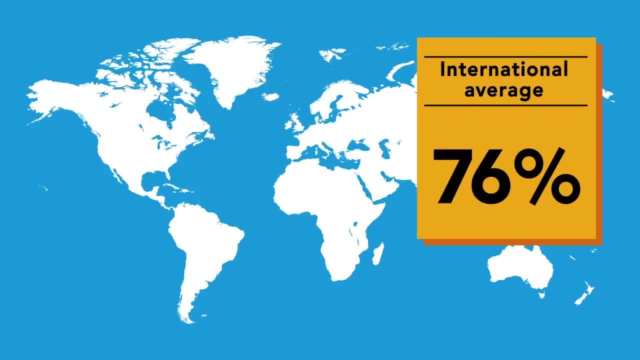 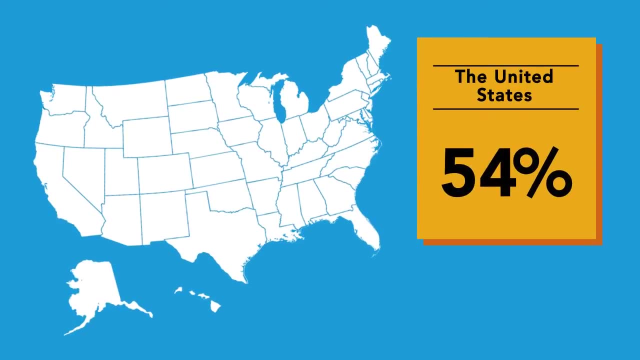 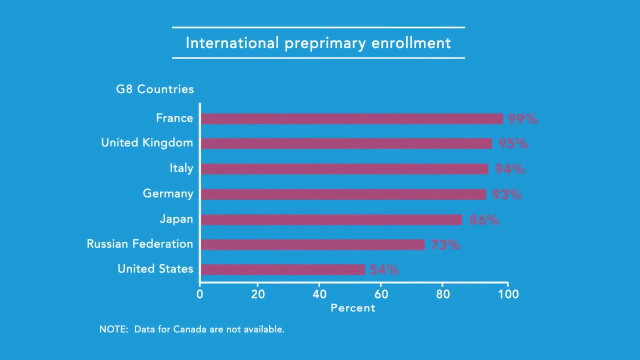 pre-school programs. In 2012,, among the 34 Organization for Economic Cooperation and Development countries, an average of 76% of three and four-year-olds were enrolled in preschool programs, compared to 54% in the United States. Enrollment percentages ranged from 12% in Turkey to 99% in France.